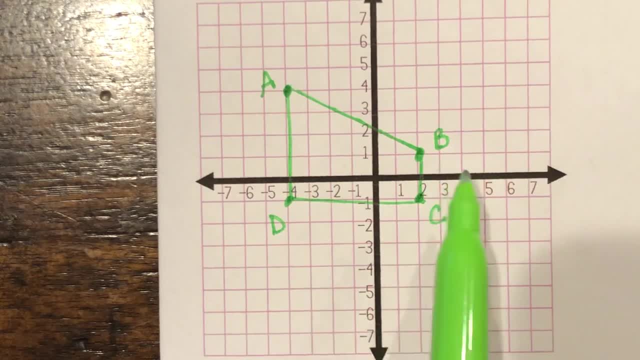 this figure. we know that we have all straight lines except for this one. I got a little squiggly down here, but they are all straight lines and we have one, two, three, four straight lines. so that makes us a quadrilateral. what kind of quadrilateral we have? well, we have to dig in a little deeper. let's see. we have 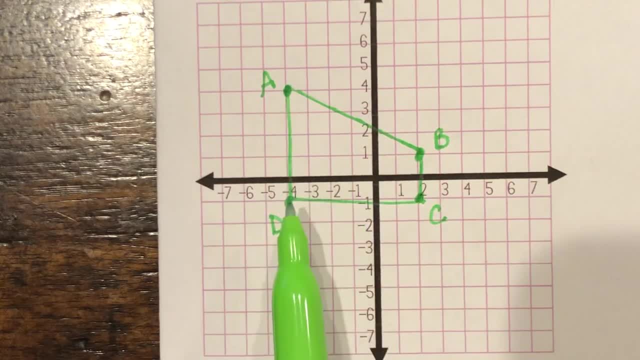 well, those are not parallel. but we do have a parallel line here and here, but these lines are not parallel. I don't have any other pairs, just line a. D is a straight line, and then we have a straight line and then we have a parallel to line BC. so for a quadrilateral that has one set of 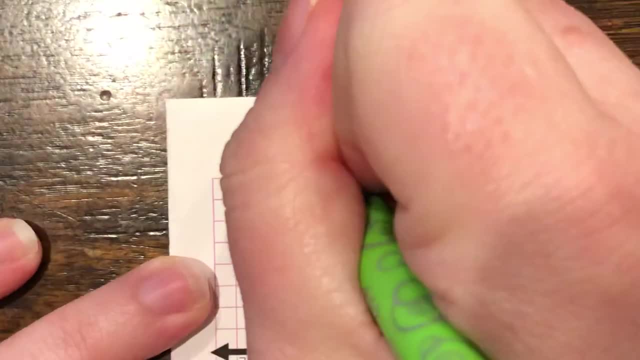 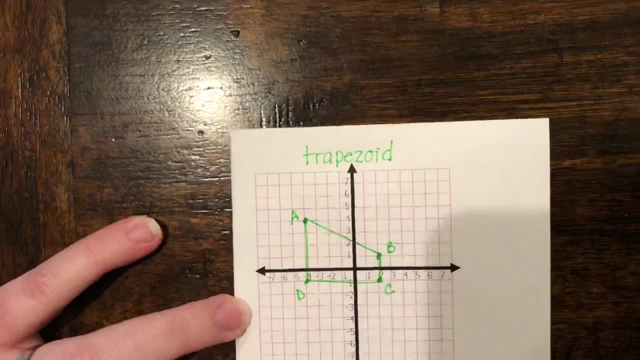 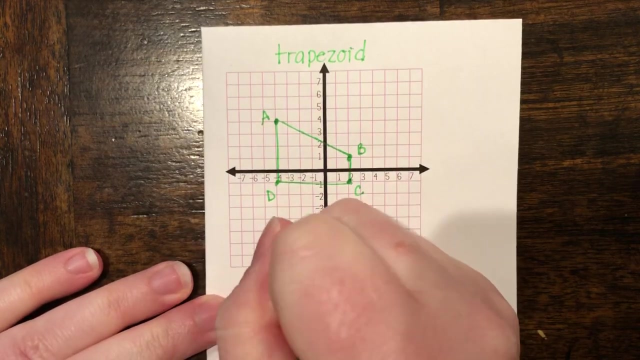 parallel lines, we have what is known as a trapezoid. so this figure is a trapezoid. now that we know what kind of figure this is, we can figure out what the area is. so let's go ahead and write: the area of a trapezoid, the area of a. 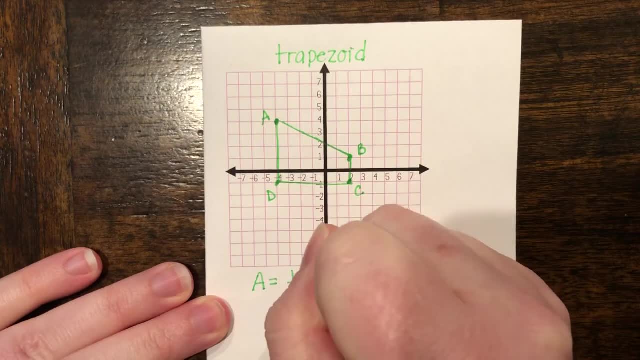 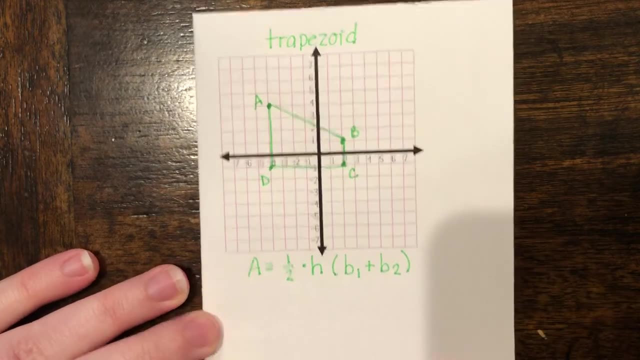 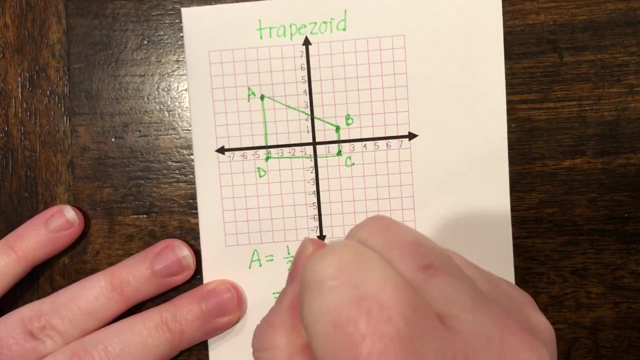 trapezoid is one half times its height, times the group of base one plus base two. alright, now that we have this formula, let's go-ahead and start plugging in what we know. alright, so we have one half times the height. now here's where I think you guys are getting mixed up. you're wanting to do. 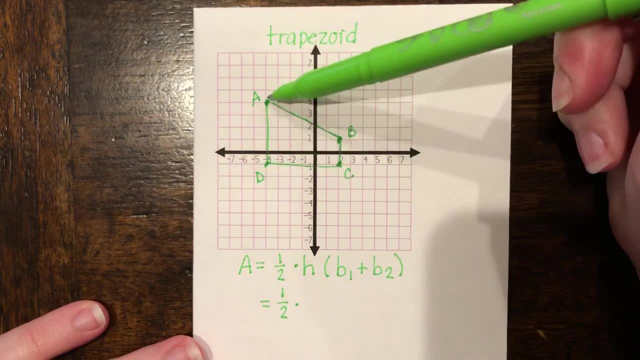 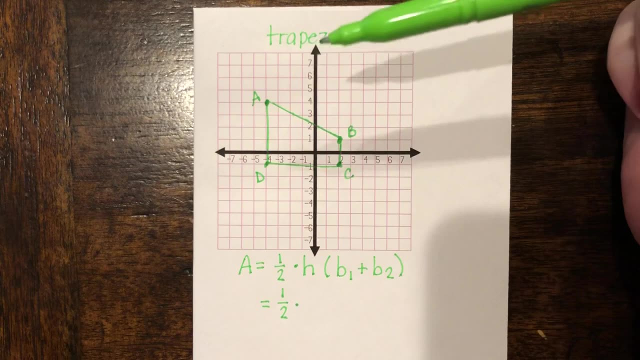 the height as this line right here to this line right here and just calculate the height here. but that's not how a trapezoid works. a trapezoids height is actually from base one to minus two and that's how a trapezoid works. a trapezoid is actuallycoins. 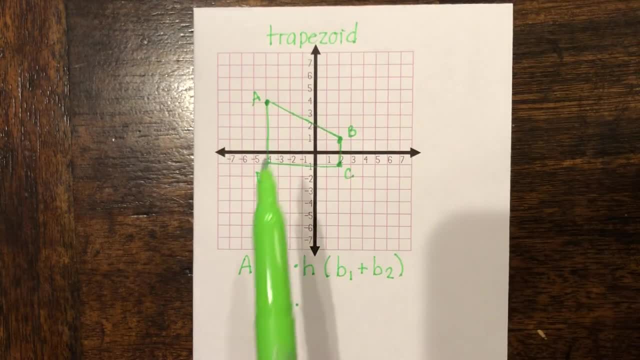 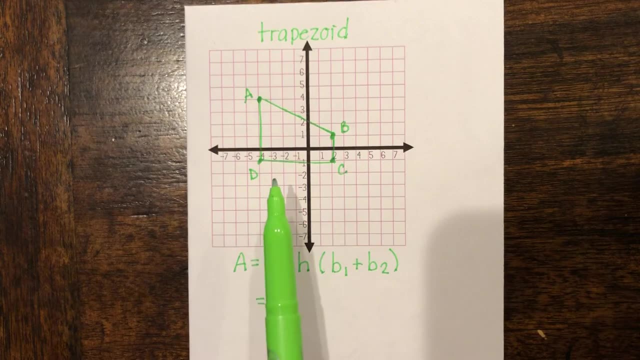 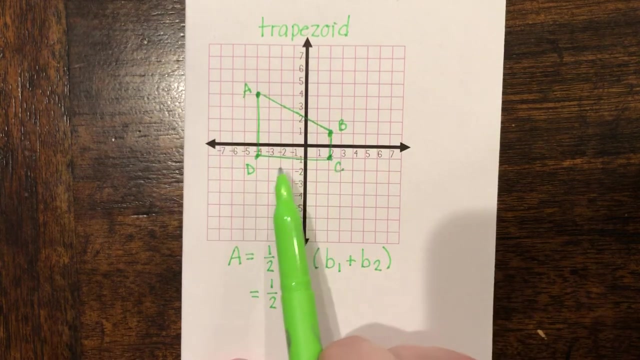 base to base. Now here's what's a little confusing, because all the trapezoids we've done so far the base has been on the bottom and the top. But if you notice in this figure our bottom line and our top line are not parallel to each other. So these lines right here are not our bases. They 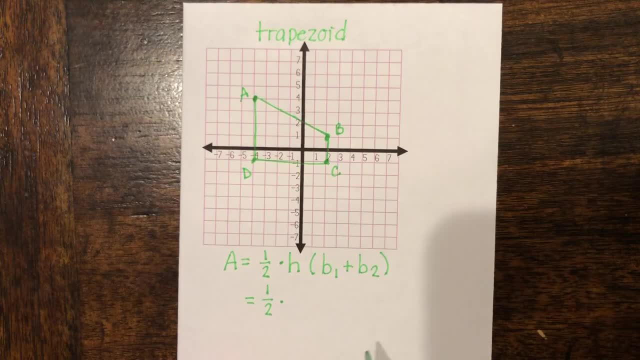 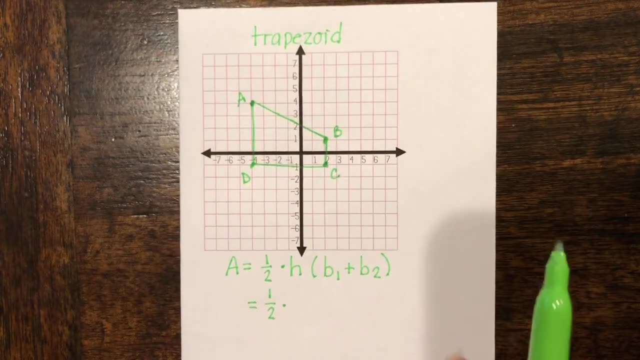 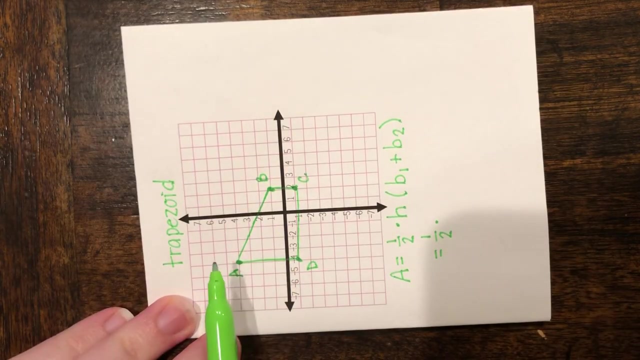 are actually the legs of our trapezoid. The bases are actually the parallel lines AD and BC. Now here's a little trick: If you're having a really hard time with that, just turn your coordinate plane and now it looks more like the problems that we've done so far, where we have our bases. 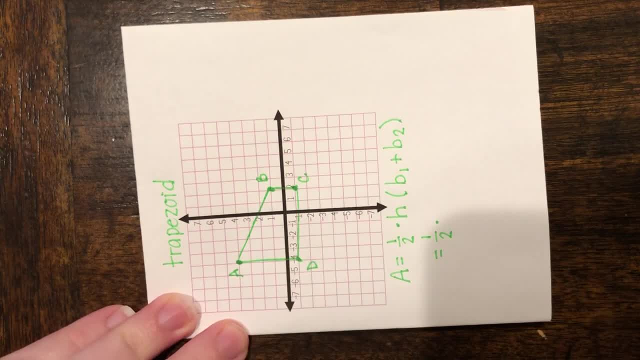 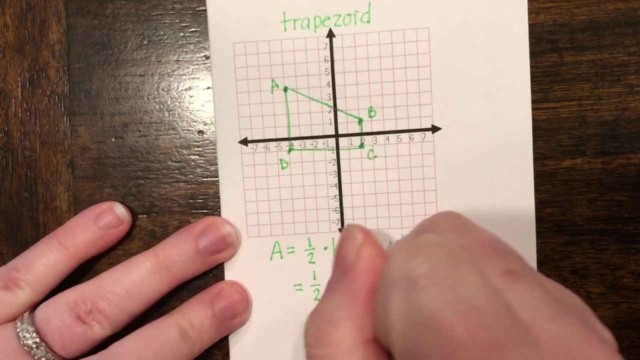 on the bottom and the top. So now that we know that the height is from base to base, let's go ahead and count how many units it is from base to base. So let's start here in the bottom on AD and we'll go 1,, 2,, 3,, 4,, 5,, 6.. So we have 6 units. So our height for this trapezoid is 6.. 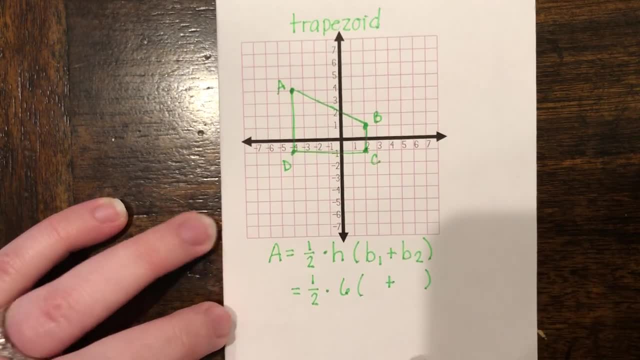 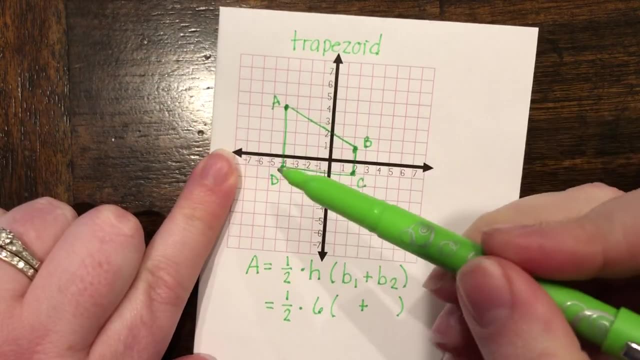 All right, Now let's see what our bases are. Again, I'm going to go ahead and turn it. If you don't want to turn it, if you know that these two are your bases, you can go ahead and start counting right here for your bases. But I'm going to move it back, just for those who need that extra. 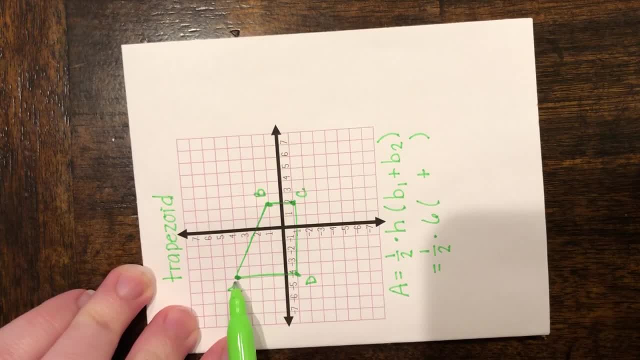 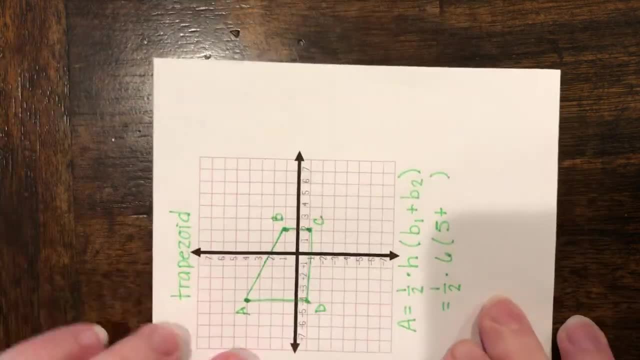 visual there. So I'm going to do line AD for the first base. So we've got 1,, 2, 3,, 4, 5 units And now I'm going to do our other base on the top line BC, And we have 1,. 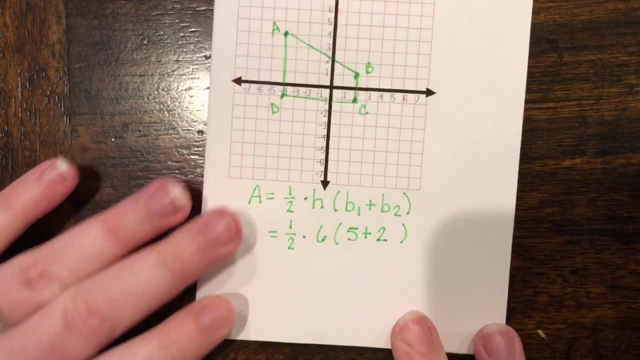 2,, 3,, 4,, 5 units. And now I'm going to do our other base on the top line BC, And we have 1,, 2,, two units, And now we just need to solve our equation. So let's go ahead and bring down our 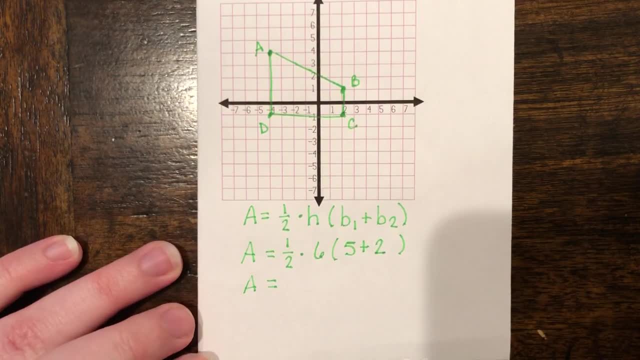 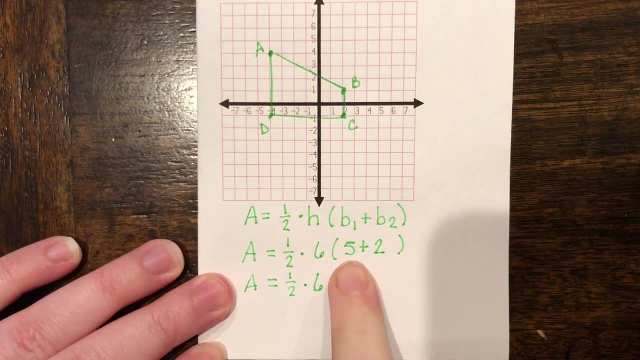 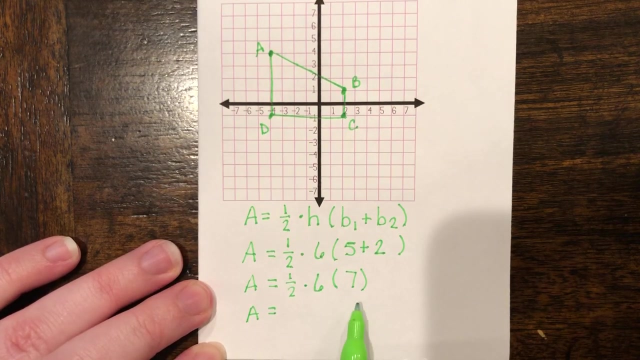 area equals PEMDAS. orders of operations tells us that we need to do what's in the parentheses first, So let's go ahead and do that. So we have one half times six, five plus two, which gives us seven. We're going to keep on moving down the line. Now we have one half times six times seven. 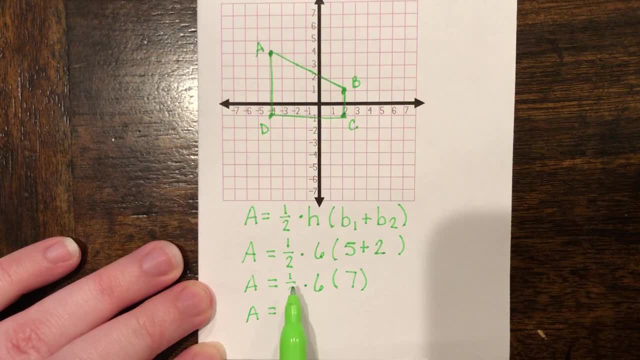 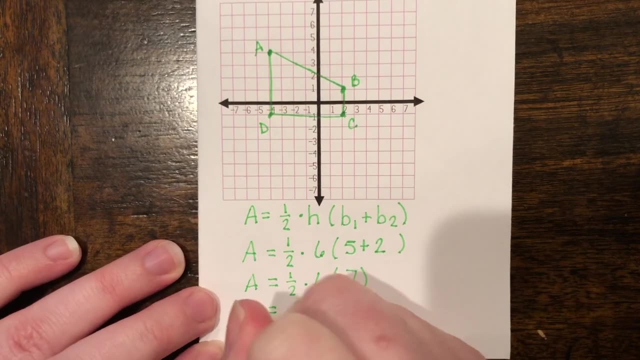 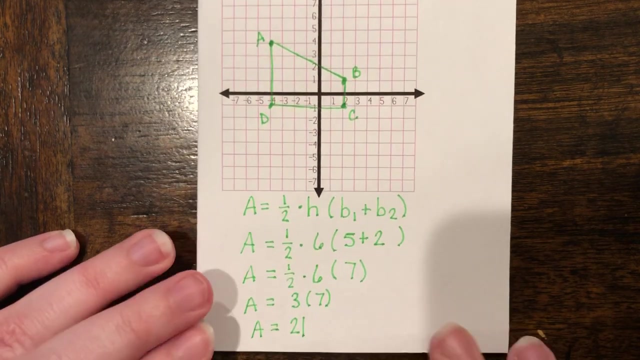 We have to do this set of multiplication first. So we have one half times six, which gives us three. Bring down the rest of your equation. And then, lastly, we have three times seven, which gives us 21.. Now, when you go back into the problem, 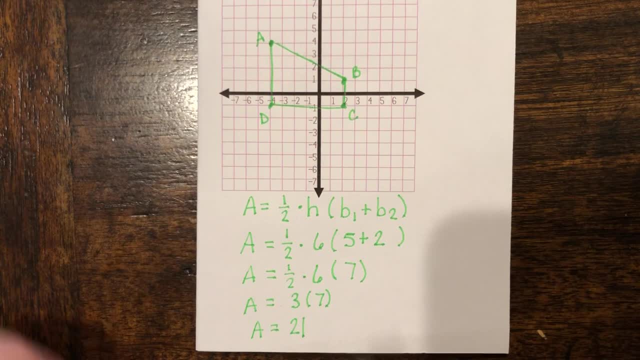 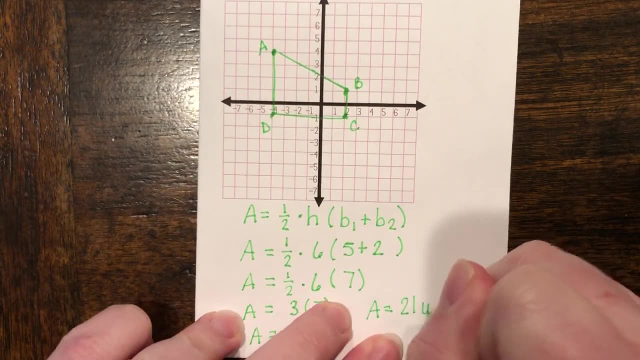 it does not say what unit this figure is, So we don't know the unit. So, in order to properly write this, we're going to say that the area equals 21 units, because it doesn't specify what units they are And we know that the area is always squared.